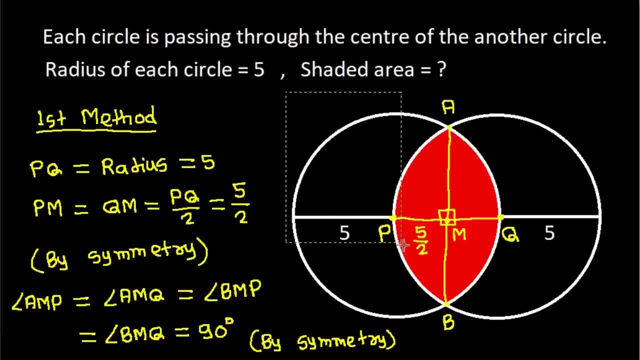 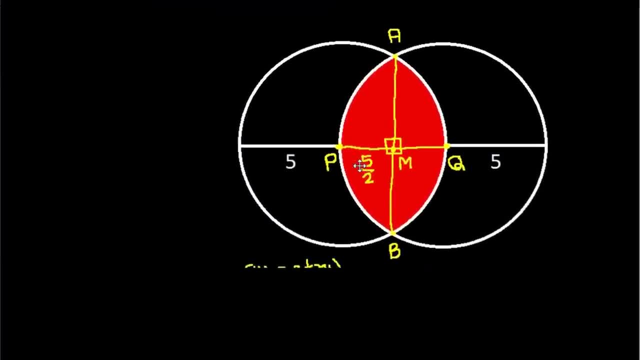 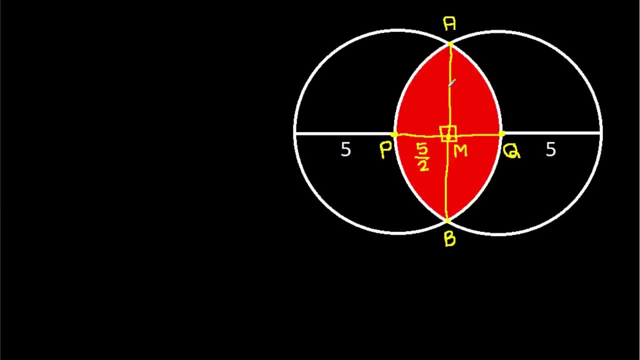 degree. and now, if we join AP, then AP it will be radius that will be five. and if we join AP, then it will be radius that will be five. AP is 5. and now inter angle AMP. it is AMP. this angle is 90 degree, AP is 5 and PM is. 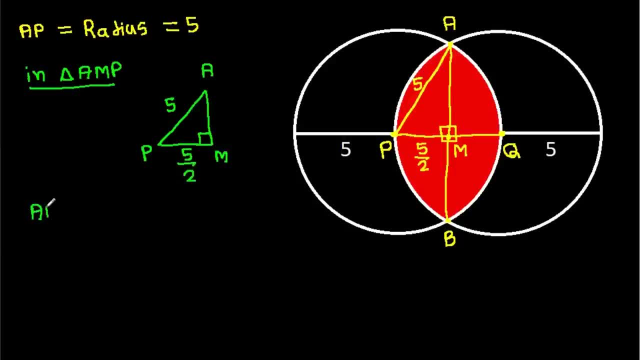 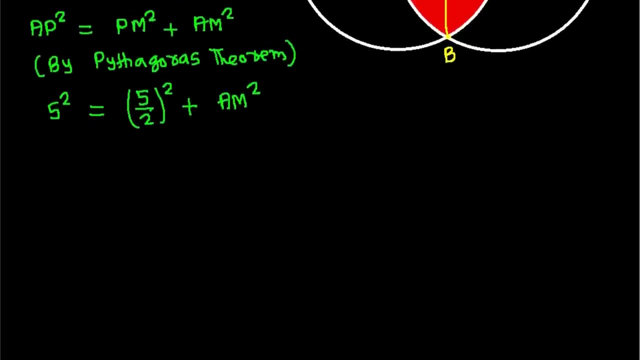 5 by 2 and AP square, it will be PM square plus AM square by Pythagoras theorem. and AP is 5 square, it is equal to PM, is 5 by 2 square plus AM square and it is 25, is equal to 25 by 4 plus AM square, So AM. 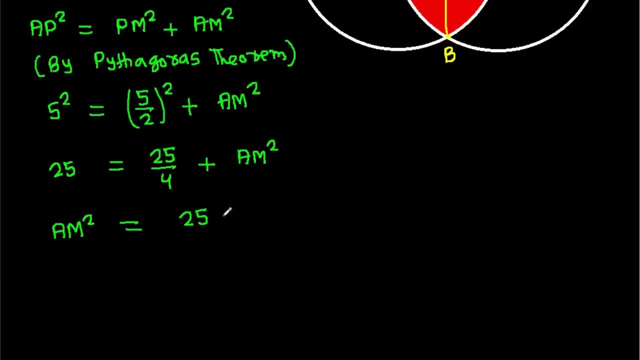 square it will be 25 minus 25 by 4.. And AM square it is equal to 100 minus 25 by 4, that will be 75 by 4.. So AM it will be equal to a square root of 75 by 4, that will be 5 by 2 times a square root of 3.. 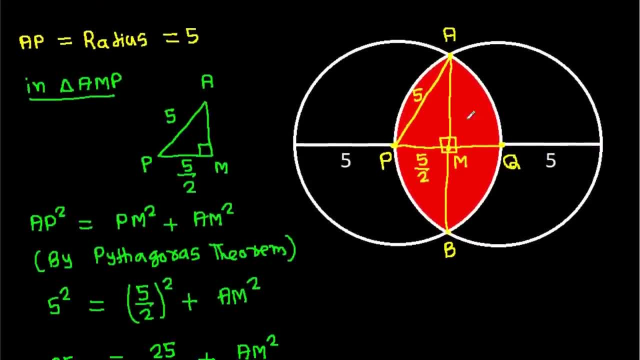 So we get AM. It is 5 by 2 times a square root of 3, and AM it will be equal to BM by symmetry. So hid it will be 5 and a square root of one third times a square root of 2 plus A. 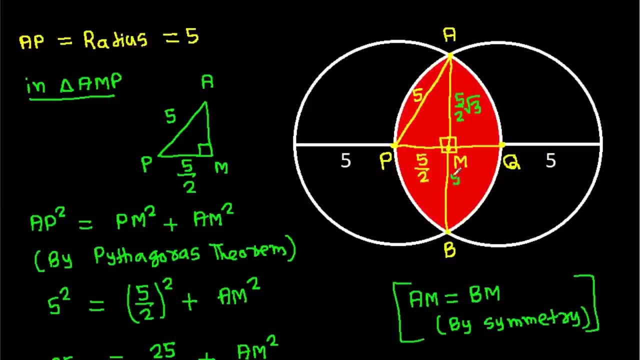 square root of one third. So it will be 5 by 2 times a square root of 3.. No AM, it will be equal to PM by symmetry. So 8 by 3 equals to 5. but transpose andило muile is comptroller. 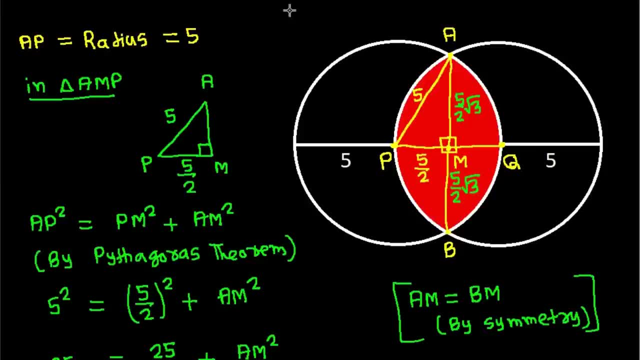 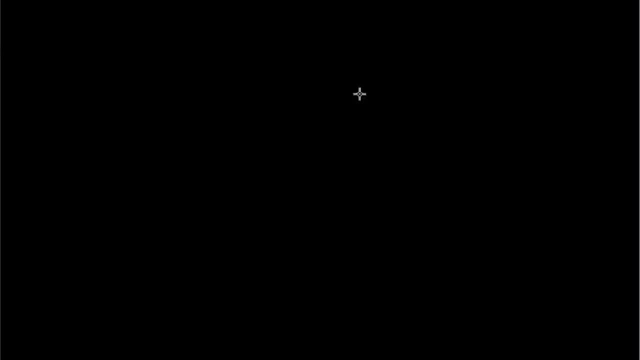 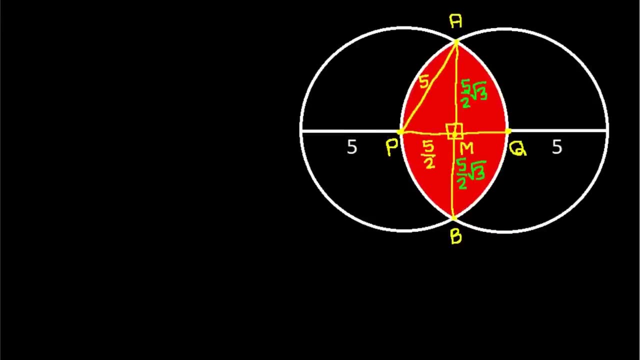 a square root of 3 and now inter angle AMP, it is A M, P. this angle is 90 degree, PM is 5 by 2, AP is 5, and suppose this angle is theta, then cos theta it will be PM by AP and cos theta. 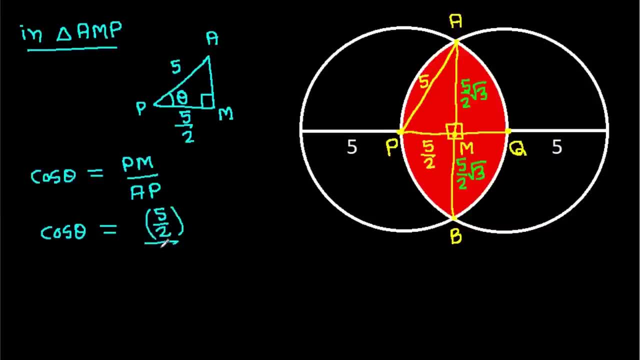 it is 5 by 2 by 5 and that will be 1 by 2, and cos theta is 1 by 2. that means theta, it will be 60 degree, and angle APM it will be equal to angle BPM, that will be 60 degree. 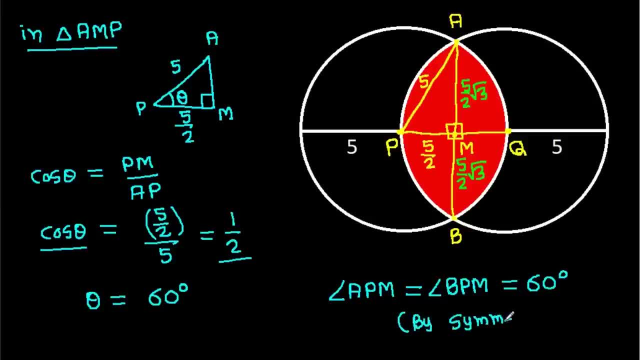 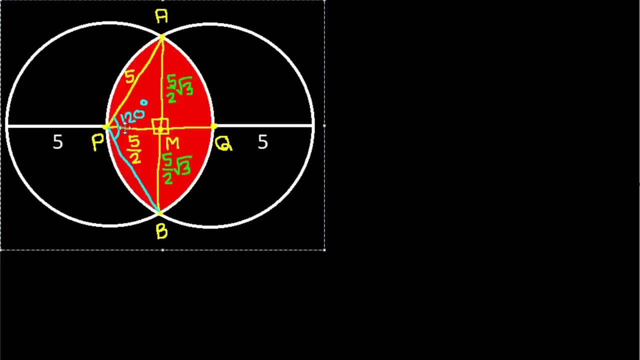 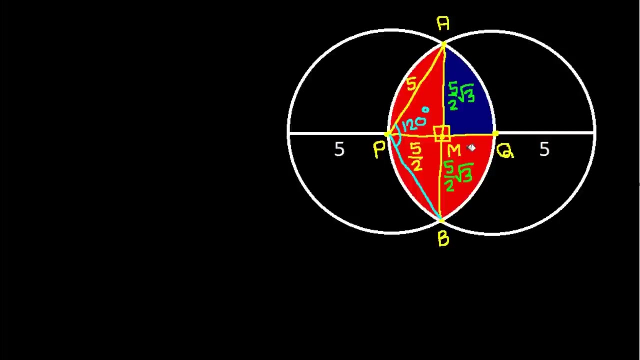 by symmetry. so if we join BP, then this angle it will be 60 degree minus 60 degree, that will be 120 degree. and now Suppose this is blue area and this is green area, then blue area it will be equal to blue plus green area, minus green area. 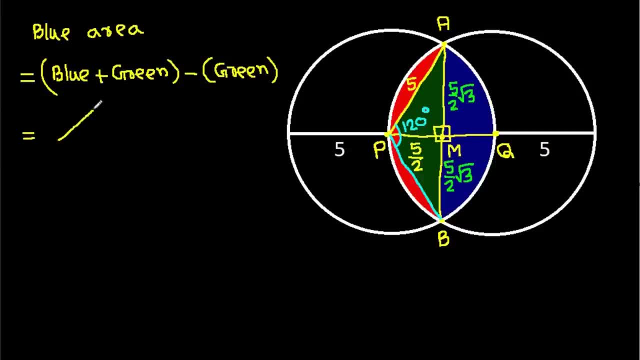 And blue plus green area. it is area of a sector of circle and this angle is 120 degree and radius is 5.. minus green area, it is area of a triangle: PAB and AB. it is 5 by 2 s square root of 3, minus. 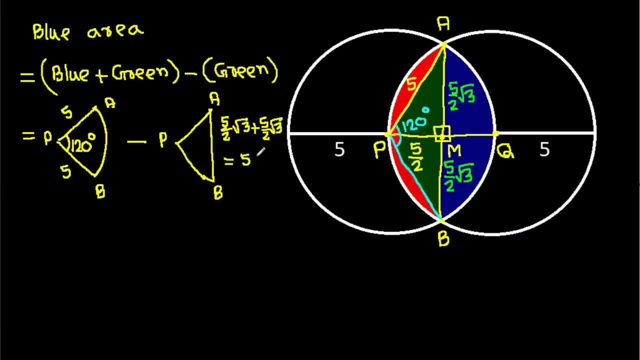 5 by 2 s square root of 3, that will be 5 times s square root of 3.. And height it is 5 by 2, so this area it will be 5 times radius, is 5 s square and angle. 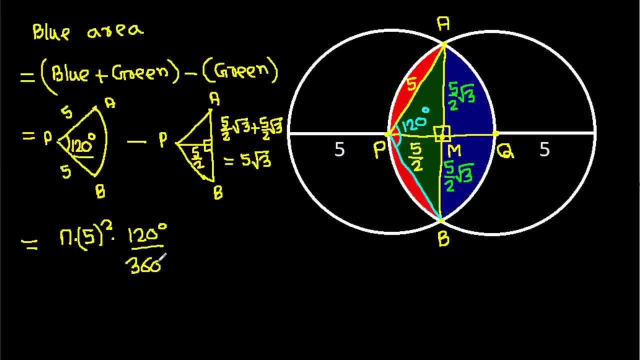 is 120 degree by 360 degree, minus this area, it will be 1 by 2 times base is 5 times s square root of 3.. What is the value of radius and height is 5 by 2 and 120 times 3 is 360.. So it is 25 pi by 3 minus 25 times a. 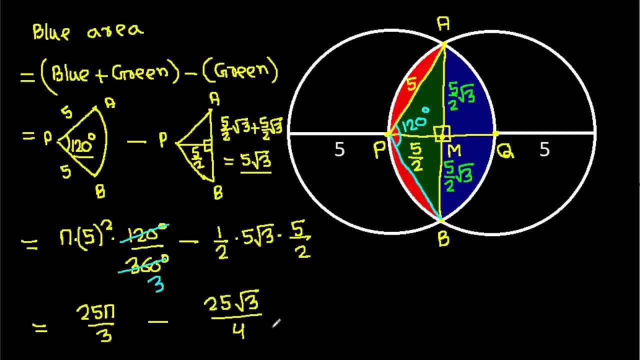 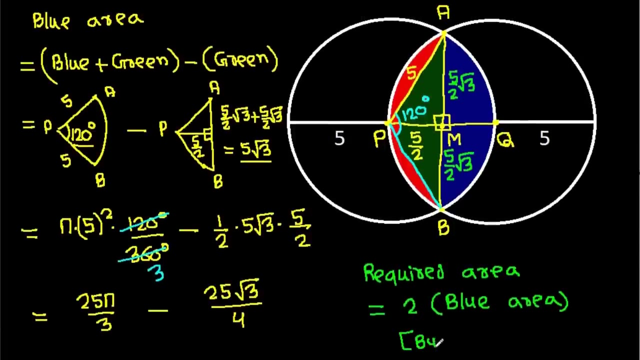 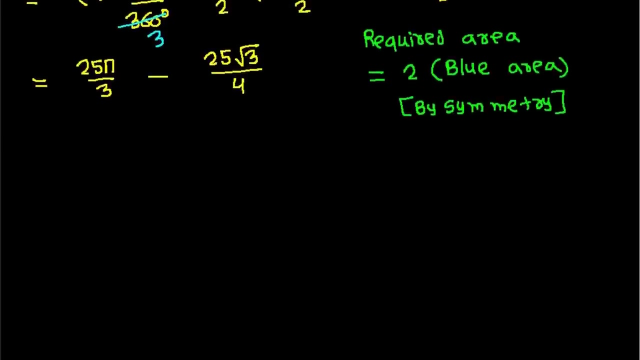 square root of 3 by 4 and required area, it will be equal to 2 times blue area by symmetry. so it will be 2 times 25 pi by 3 minus 25 times a square root of 3 by 4, and it is: 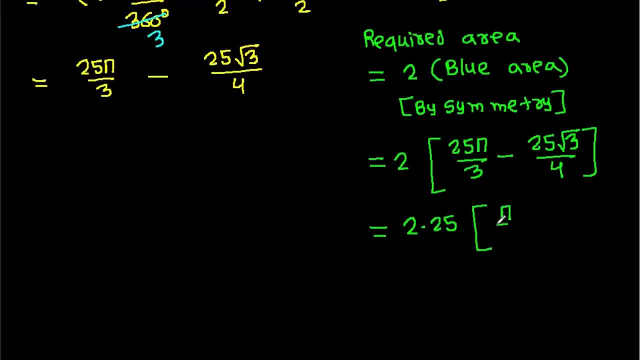 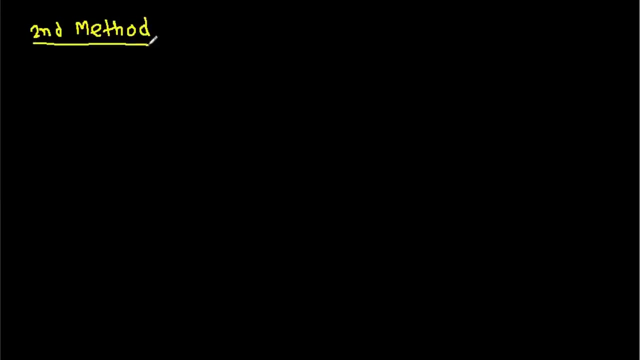 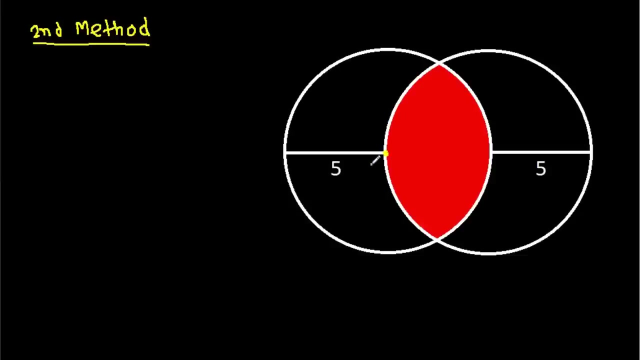 2 times 25 times pi by 3 minus a square root of 3 by 4, and it is 50 times pi by 3 minus a square root of 3 by 4. and the second method, this point is p. this point is q. 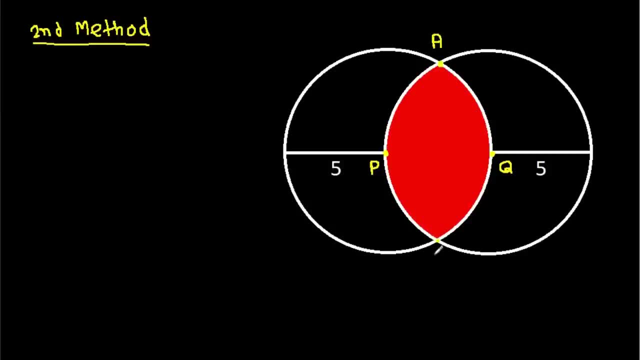 this point is p, this point is q. this point is p, this point is q. this point is a and this point is b. this point is a and this point is b. this point is a and this point is b. and if we join pq and if we join pq. 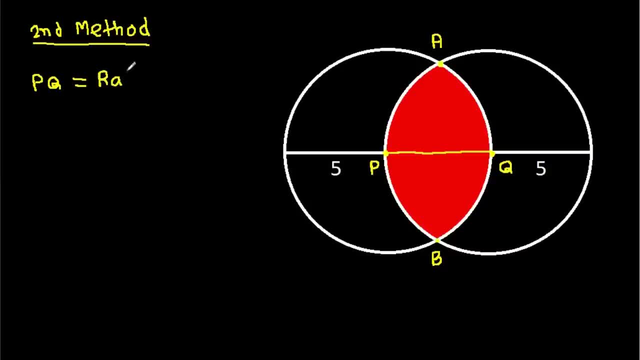 and if we join pq, then pq it will be radius, then pq it will be radius, then pq it will be radius. that will be 5. if we join pa, that will be 5. if we join pa, that will be 5. if we join pa and qa. 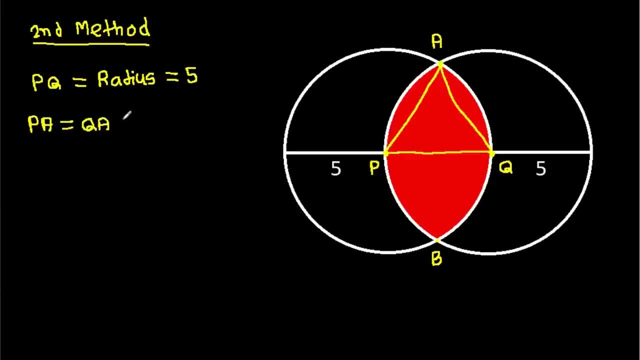 then qa, then pa, then qa, then pa. it will be qa that will be radius, so it it will be qa that will be radius, so it it will be qa that will be radius, so it will be 5, and now inter angle apq it is will be 5, and now inter angle apq it is. 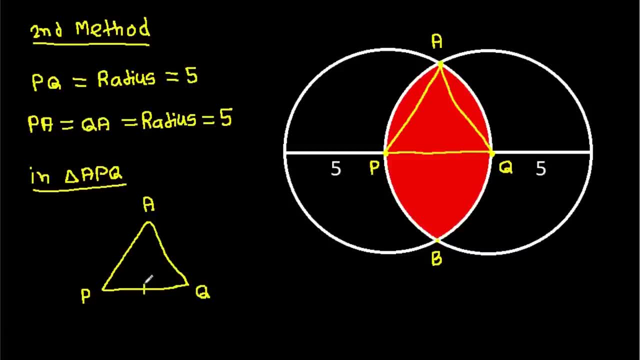 will be 5. and now inter angle: apq. it is a P, Q, P, Q. it is equal to a P. it is a P, Q, P, Q. it is equal to a P. it is a P, Q, P, Q. it is equal to a P. it is equal to a Q. that is 5. 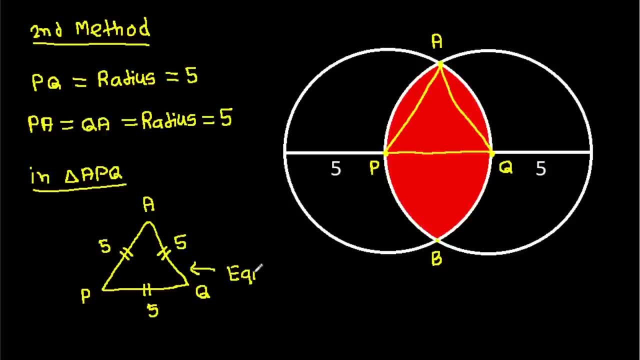 equal to a Q that is 5. equal to a Q that is 5, that means it will be equilateral. that means it will be equilateral, that means it will be equilateral triangle. so these angles, they will be 60 degree. so these angles, they will be 60 degree. 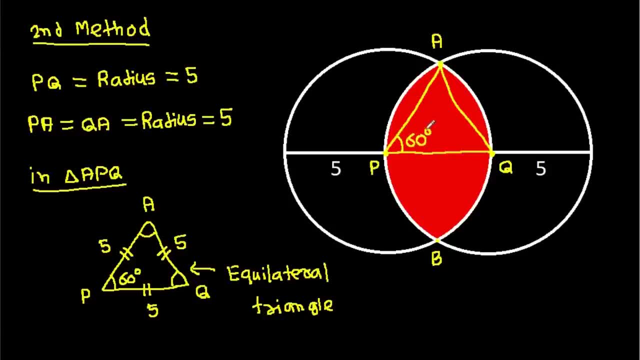 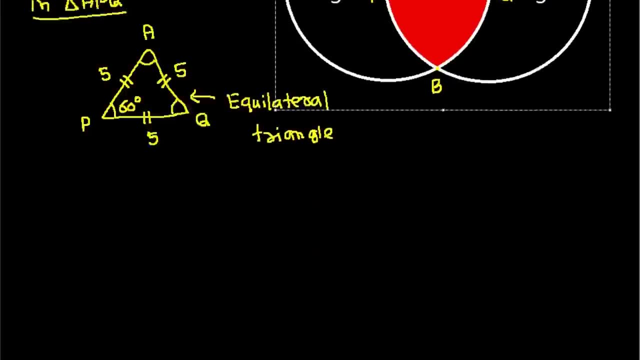 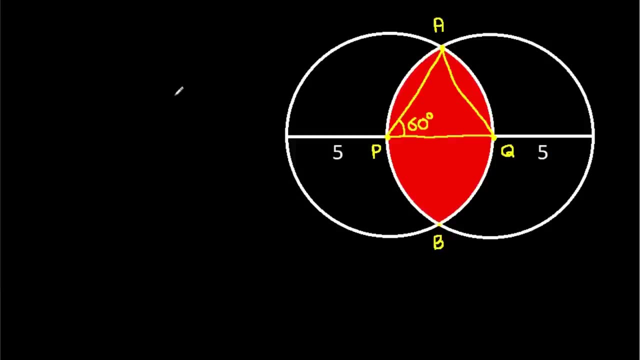 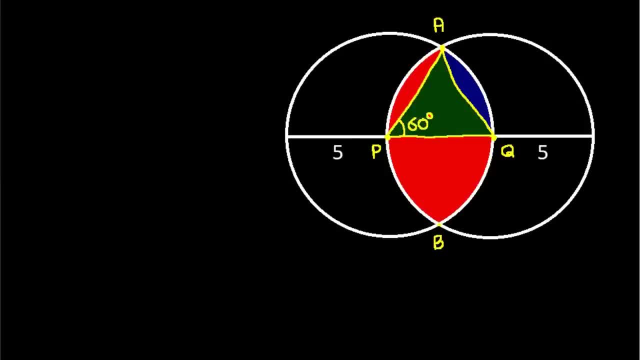 now suppose this is blue area and this is now suppose this is blue area and this is green area, then green area. it is area green area, then green area. it is area green area, then green area. it is area of a triangle, a, P, Q, whose side is: 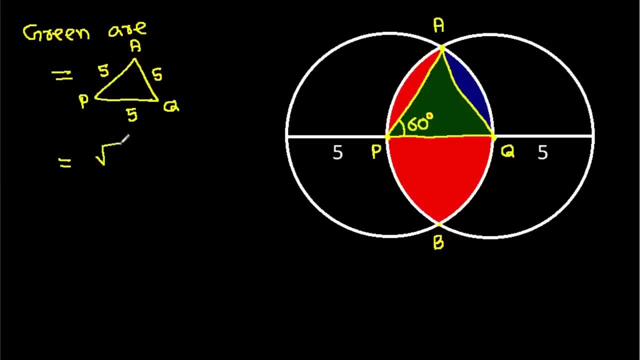 of a triangle, a P Q whose side is of a triangle, a P Q whose side is 5. so it will be a square root of 3 by 4- 5. so it will be a square root of 3 by 4- 5. so it will be a square root of 3 by 4 times 5, a square that will be 25 times a. 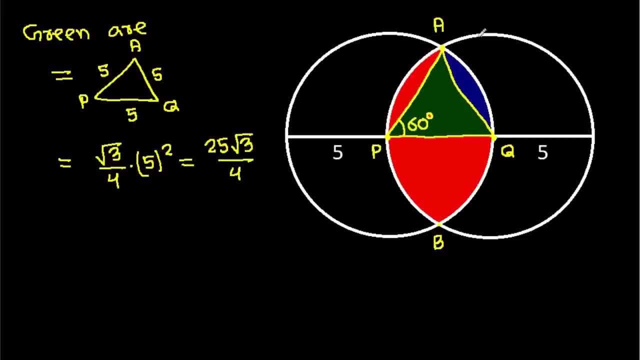 times 5 a square, that will be 25 times a times 5 a square. that will be 25 times a square root of 3 by 4. this area, it is 25. square root of 3 by 4: this area, it is 25. 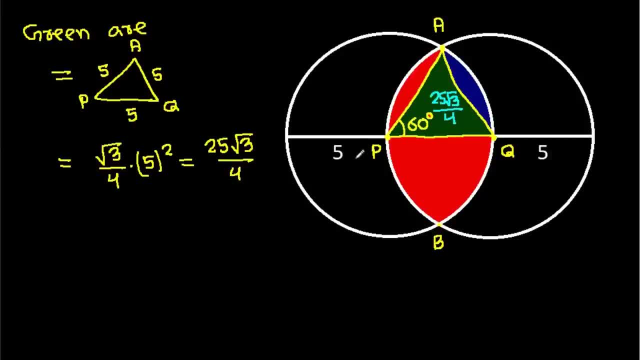 square root of 3 by 4, this area it is 25 times a square root of 3 by 4 and blue times a square root of 3 by 4 and blue times a square root of 3 by 4 and blue area, it will be equal to. 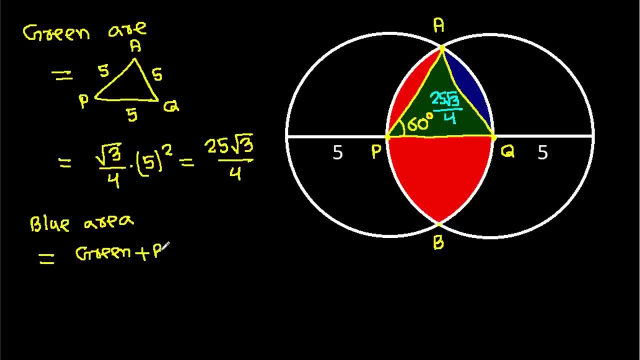 area, it will be equal to area. it will be equal to green plus blue area minus green area, green plus blue area minus green area, green plus blue area minus green area and green plus blue area. it is area of a and green plus blue area it is area of a. 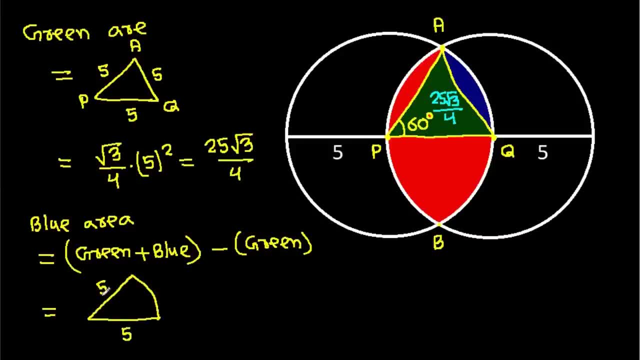 and green plus blue area. it is area of a sector whose radius is 5 and this angle sector whose radius is 5, and this angle sector whose radius is 5, and this angle is 60 degree minus green area, it is 25, is 60 degree minus green area, it is 25. 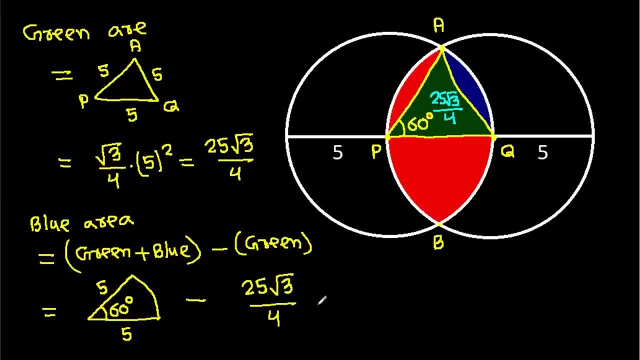 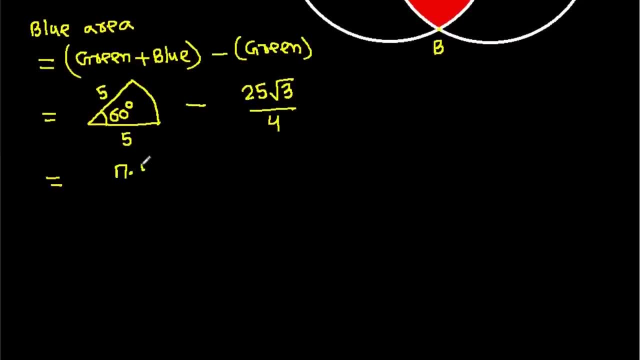 is 60 degree minus green area. it is 25 times 5 times 5 times 5, a square root of 3 by 4, and it will be pi a square root of 3 by 4, and it will be pi a square root of 3 by 4, and it will be pi times. radius is 5 a square times angle. 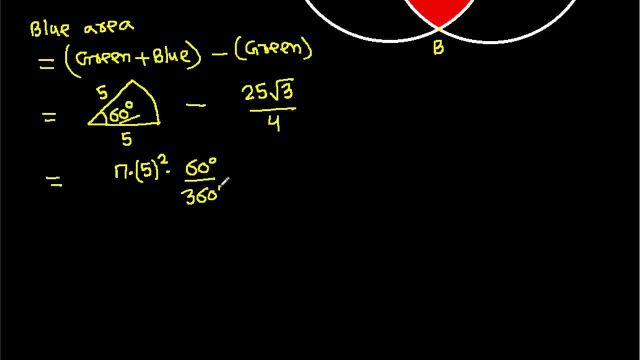 times radius is 5 a square times angle times radius is 5 a square times angle is 60 degree by 360 degree minus 25, is 60 degree by 360 degree minus 25 is 60 degree by 360 degree minus 25 times a square root of 3 by 4 and 60. 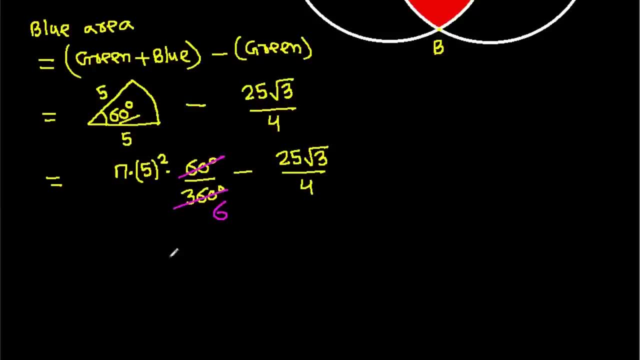 times a square root of 3 by 4 and 60 times a square root of 3 by 4, and 60 times 6 is 360 times 6 is 360 times 6 is 360. so it is 25 pi by 6 minus 25 times a. 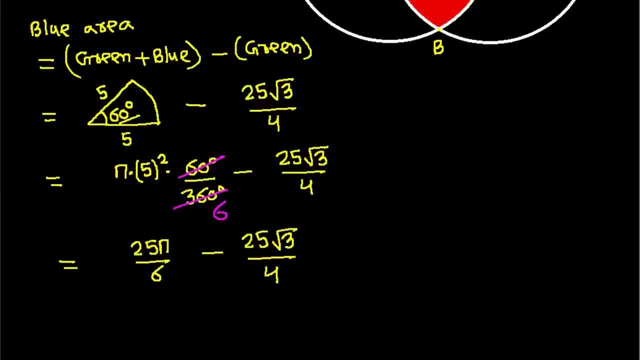 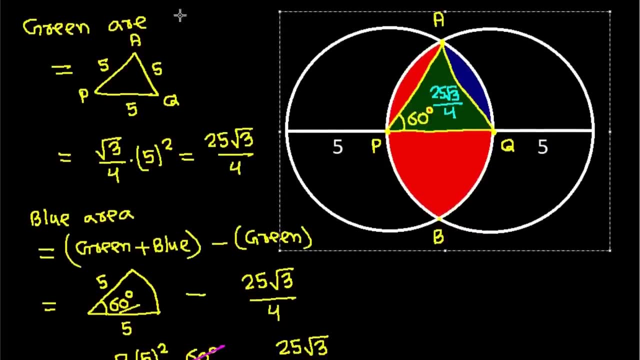 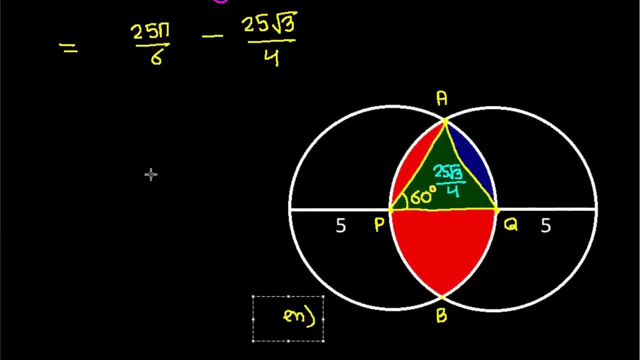 so it is 25 pi by 6 minus 25 times a, so it is 25 pi by 6 minus 25 times a square root of 3 by 4. and so it is 25 pi by 6 minus 25 times a square root of 3 by 4 and 60 times a square. 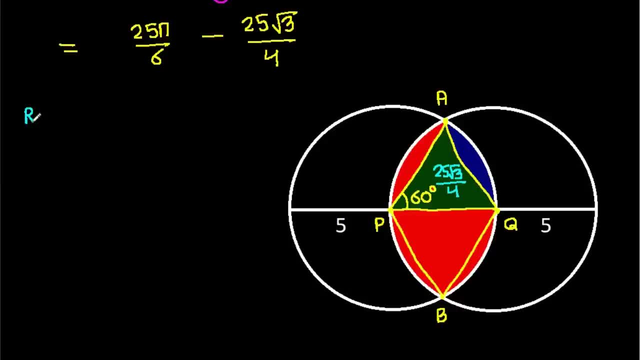 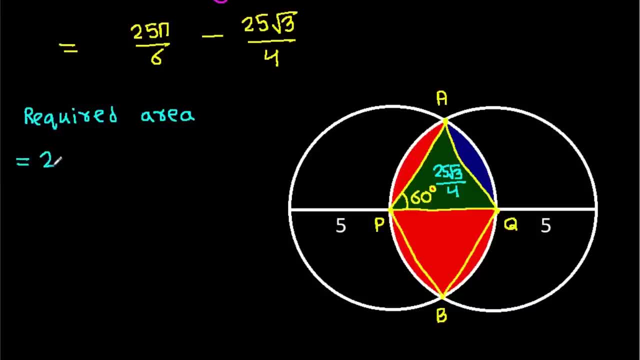 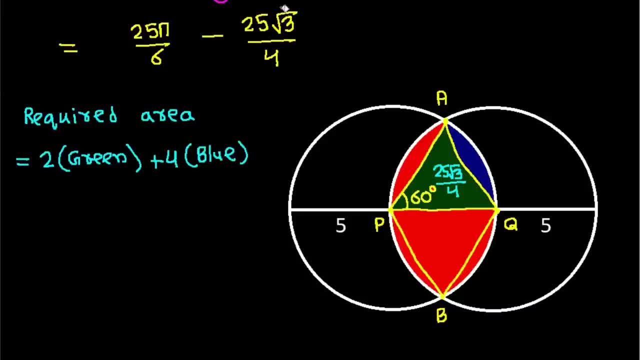 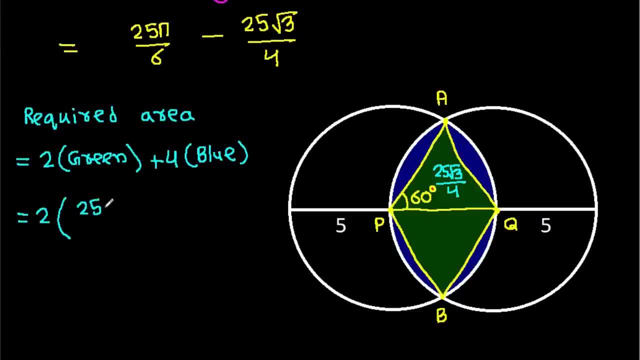 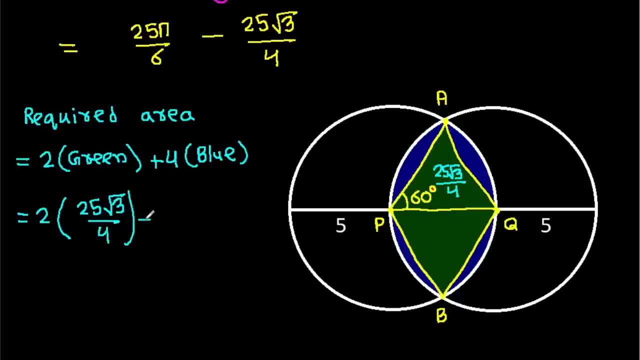 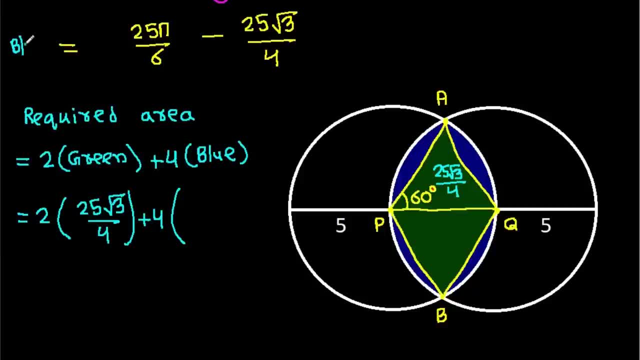 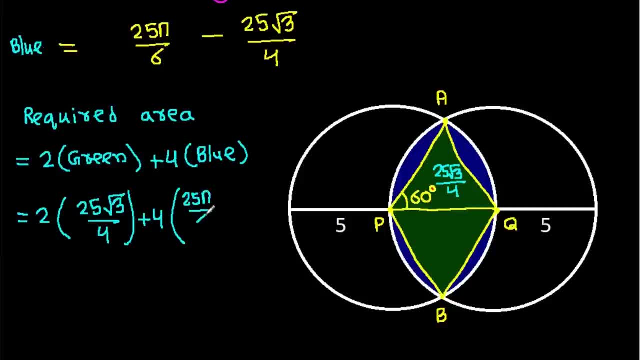 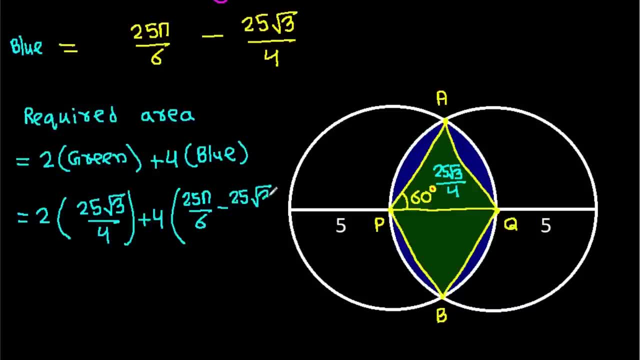 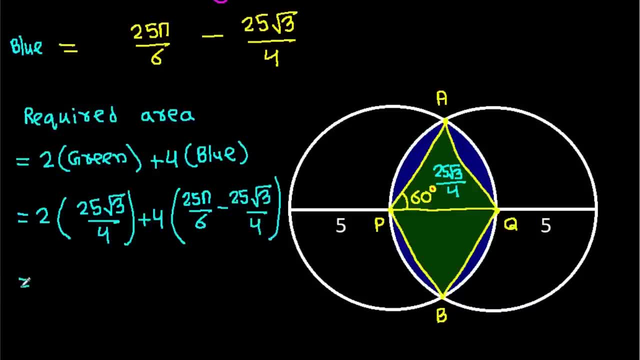 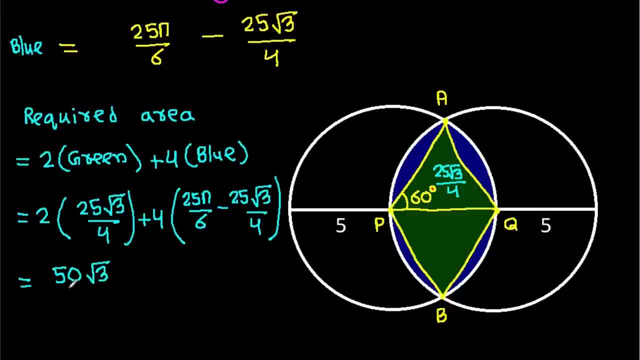 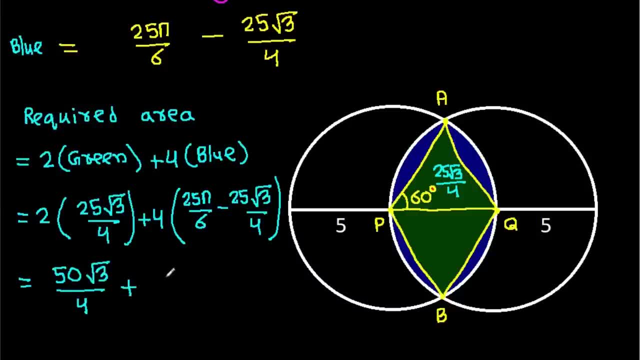 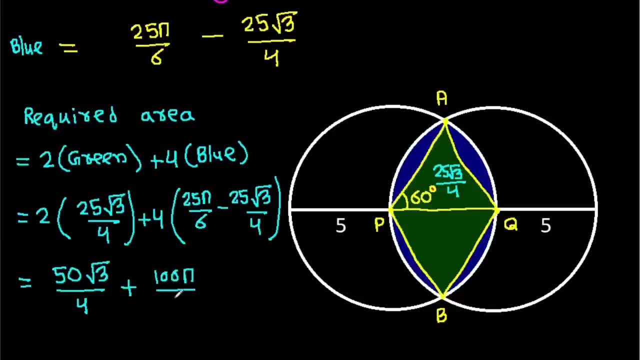 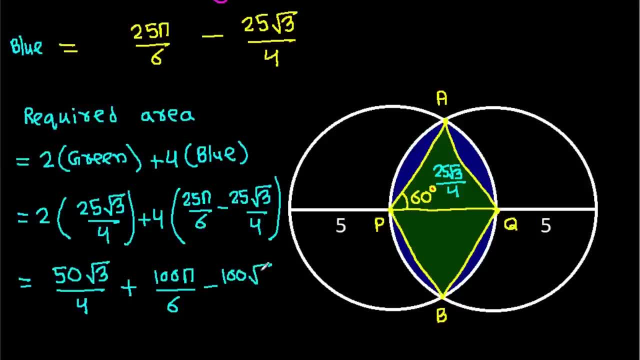 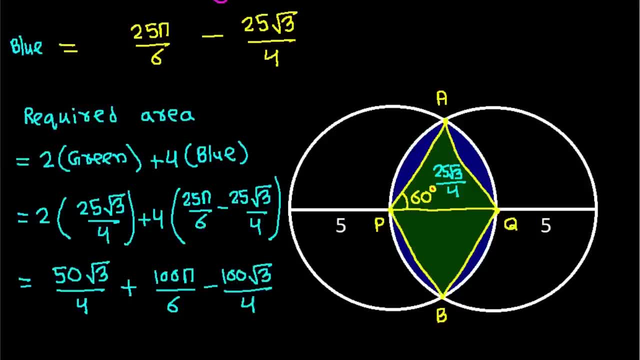 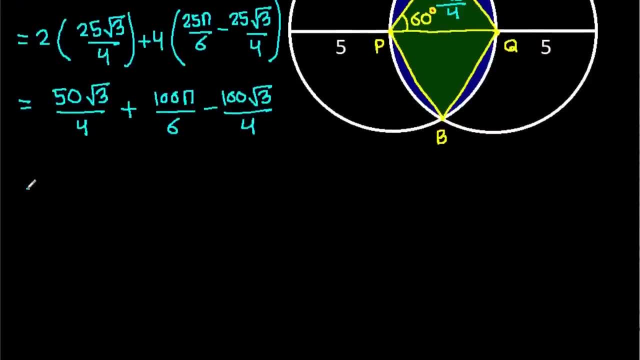 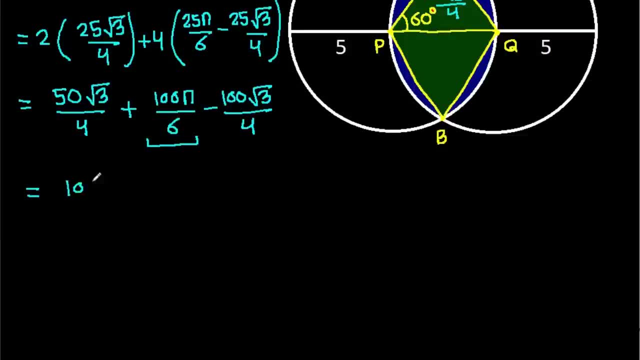 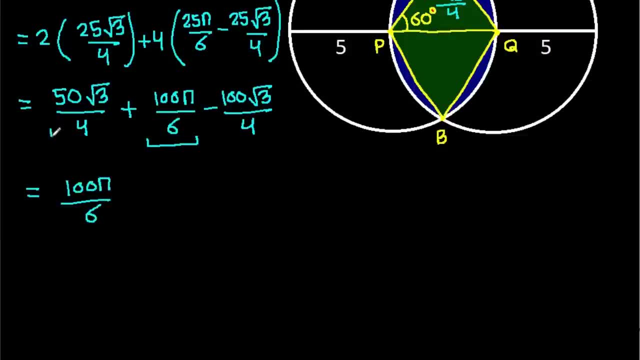 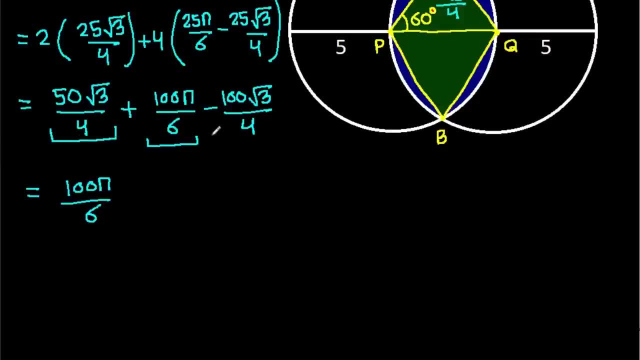 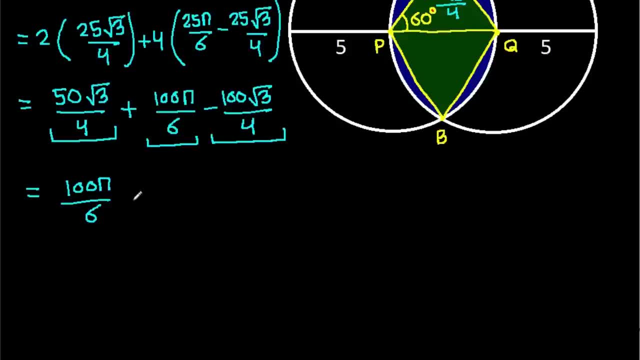 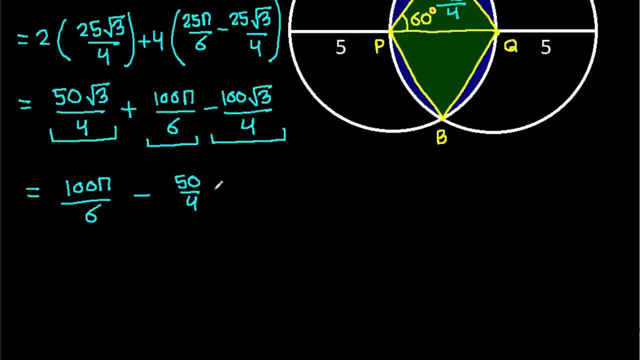 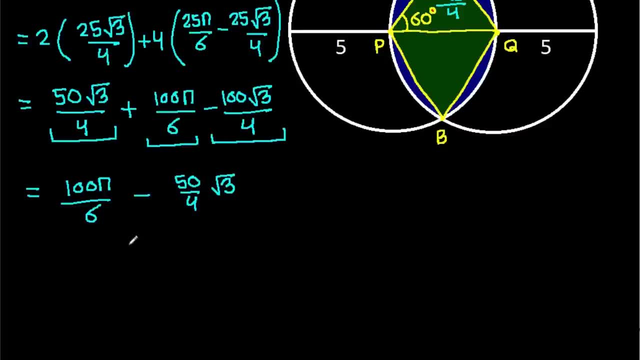 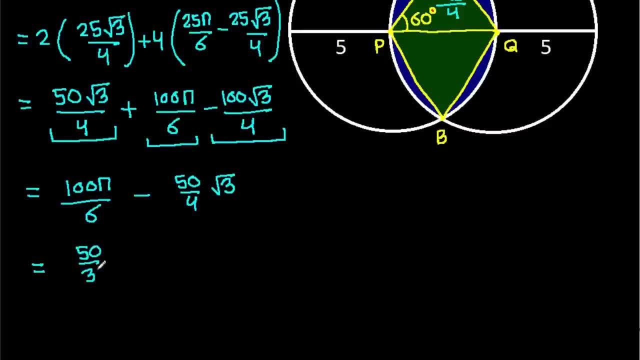 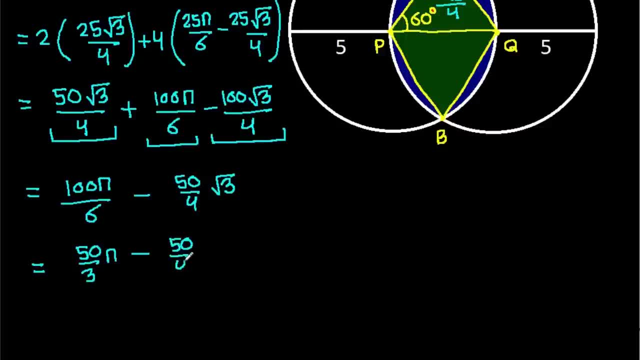 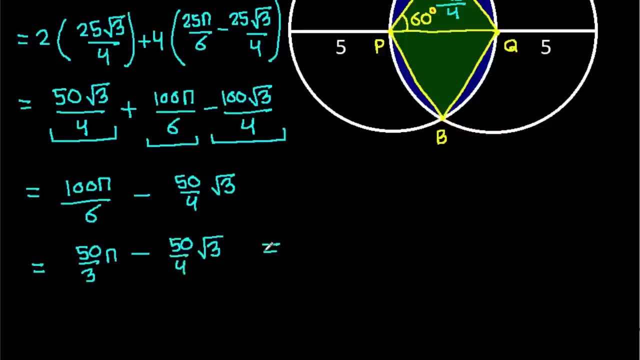 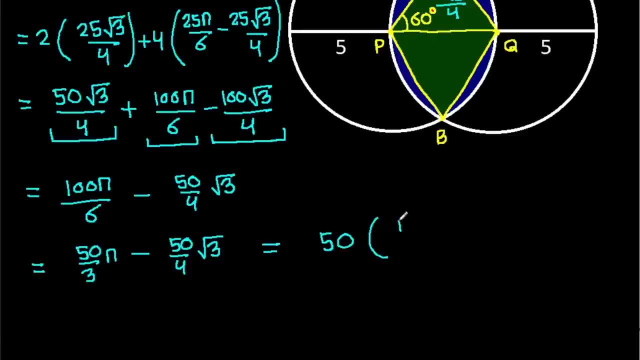 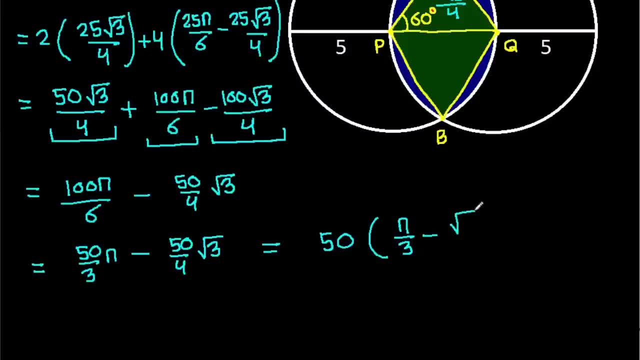 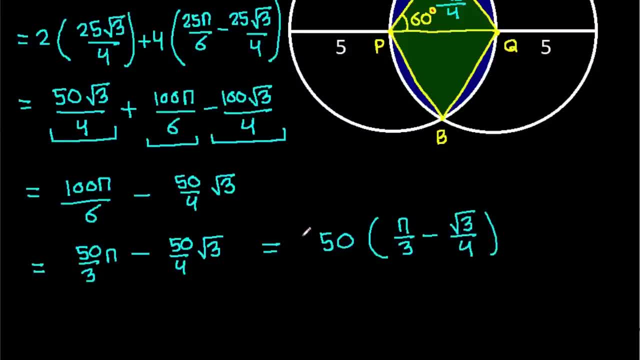 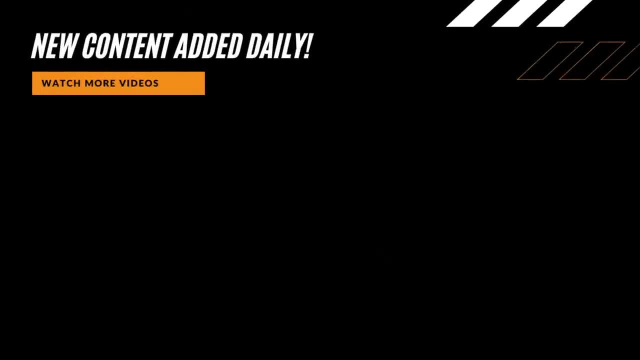 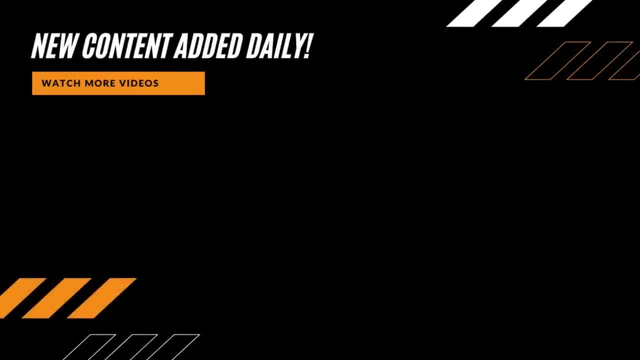 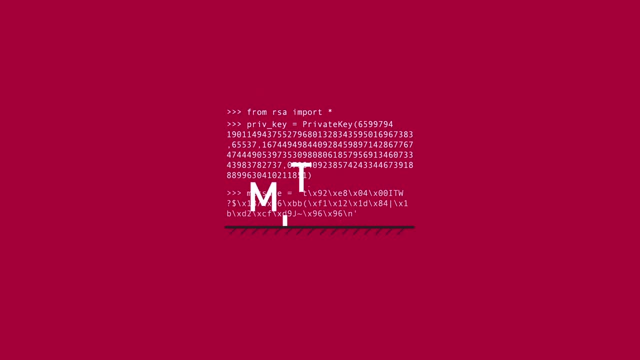 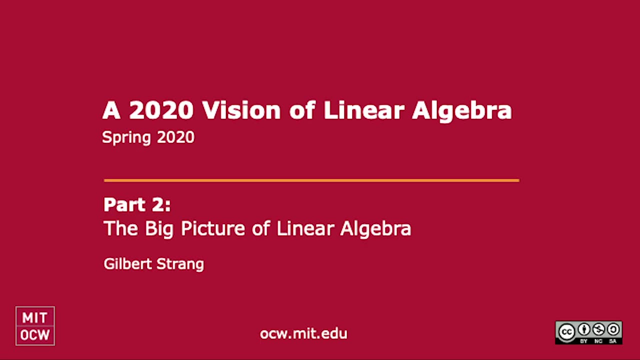 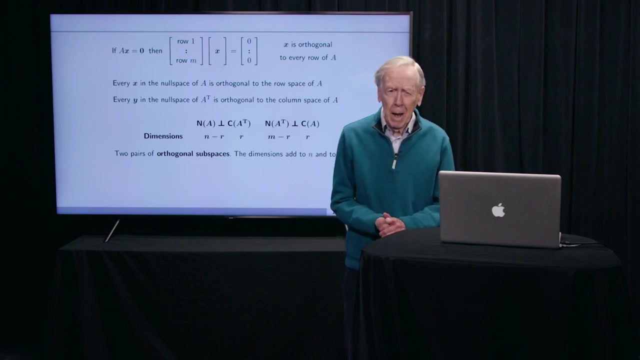 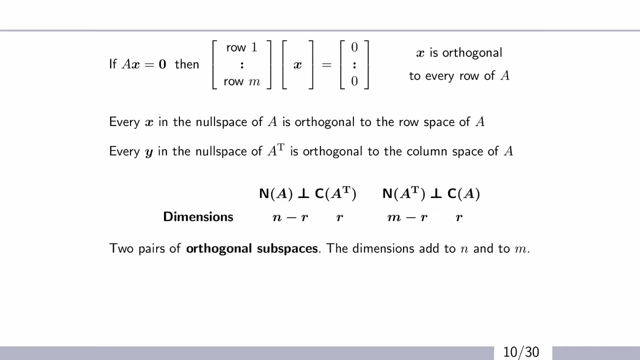 OK, In this second part I'm going to start with linear equations: a times x equal b. And you see, actually the good starting point is a times x equals 0.. So are there any solutions to the matrix, any combinations of the columns that? 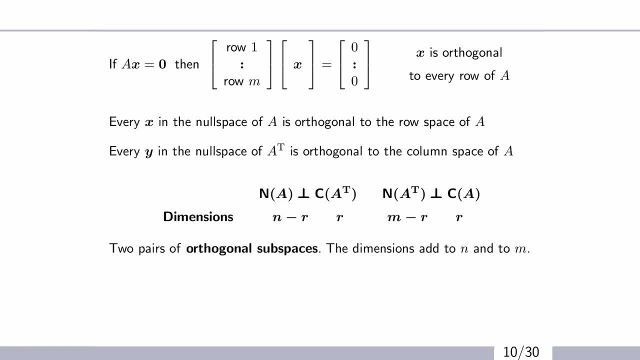 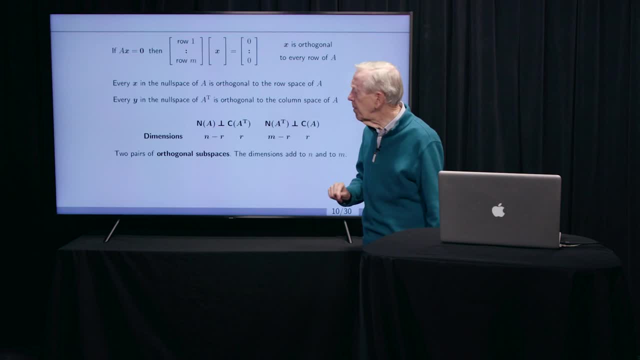 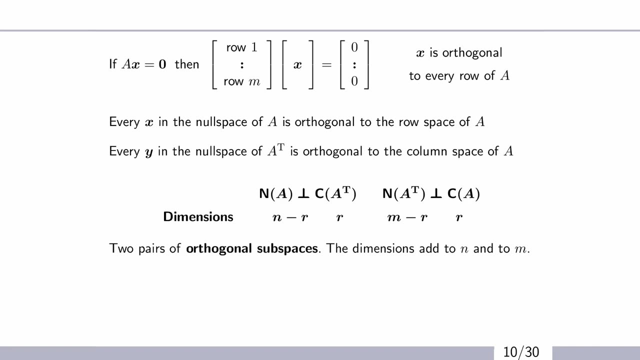 give 0, any solutions to a times x equals 0?. Now I'm multiplying a matrix A by a vector x. In the way you'll know, I take rows of x times. it's called a dot product row of x row, sorry, rows of A.